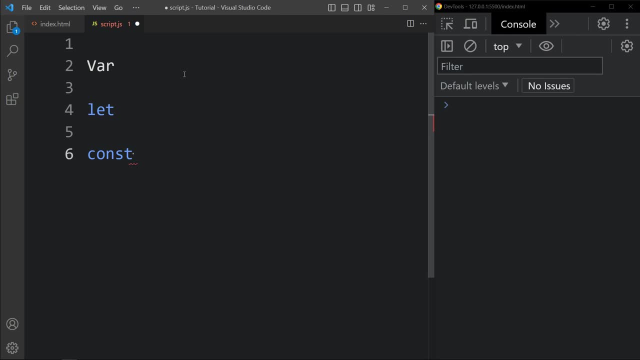 The const keyword is used to declare constants, which are variables that cannot be changed. Once you have declared a variable, you can assign a value to it using equal sign. For example, Let xi be equal to 2xv. Here I can set a variable such that heavy crush device equals 1xvar, or whatever the 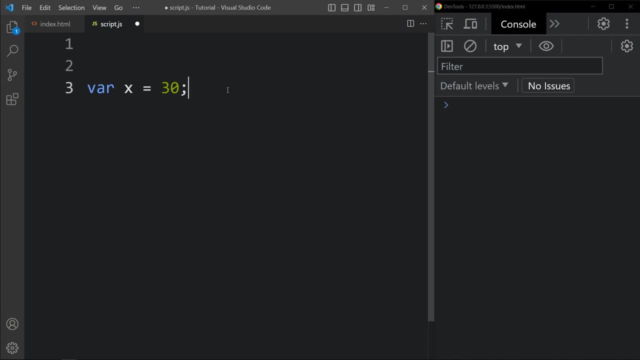 value should be. Variables can be used to store any type of data, including number, string, objects and arrays. For example, if i write var, x is equal to ב. if in, var is equal to double any message, Hello world. so here we are storing the string data type in the x variable Variables. 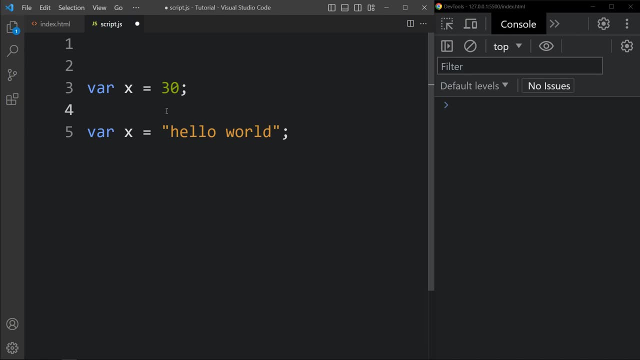 name must begin with alphabet, dollar sign or underscore. If I write 2x, it is not a valid name for the variable. If I write anything in the alphabet, it is valid and we can also declare it with the dollar sign. We can start like this: dollar x, It is valid and we can. 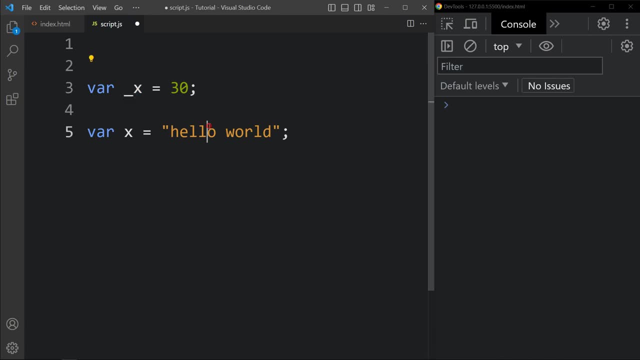 also use underscore here, like this underscore x. Let me remove it So you can see it is valid format to write a variable name. You can start with dollar and you can start with any alphabet in Uppercase or lowercase. it is valid. But if you start from the number, it is not a valid. 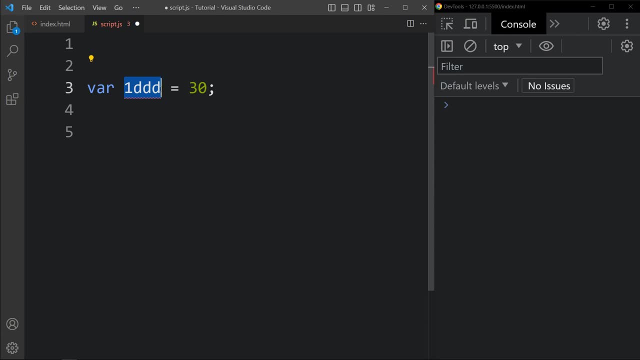 name for the variable. If you add the valid character, then later you can add number. it is valid. JavaScript is case sensitive. So if you write var first name equal to greater stack and if you write var first name with the lowercase n, So these two variables name are different. It is not. 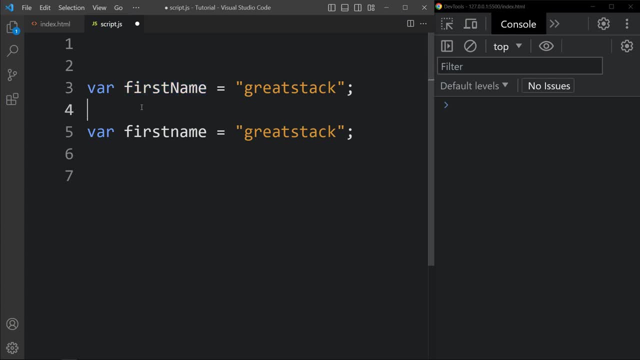 same because here we have the different case. So JavaScript is case sensitive. That's why it is two different variables name. Now let's understand about the let keyword. Let keyword in JavaScript is used to declare a block, a scoped variable. This means that the variable 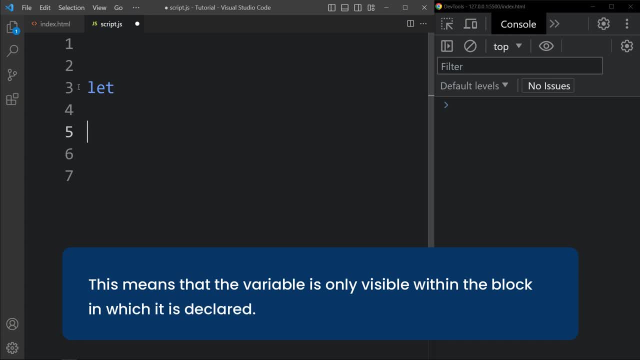 is only possible within the block in which it is declared. For example, if I write let x equal to 10 and if x greater than 5.. Yes, it is greater than 5, because the x value is 10.. In this block, 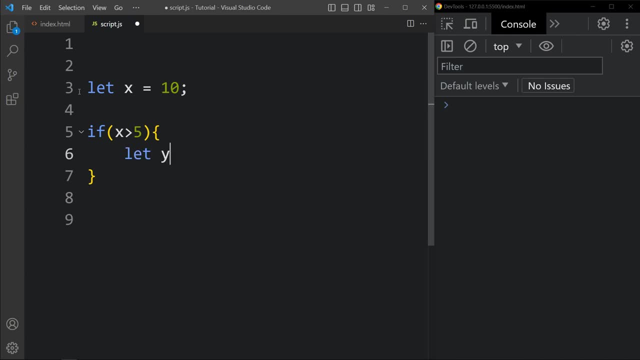 we will add let by equal to 20, and here, if i try to display the value of y, we will add console dot, log y so you can see this y value in the console tab. here you can see 20. correct, we have added this code within this curly braces, so it's a block. and if i try to access this y outside, 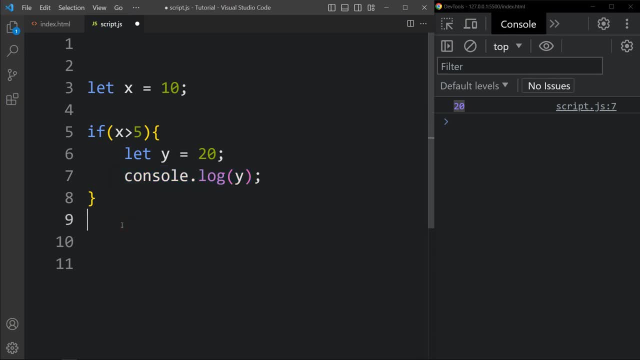 of this block. we will copy this and paste it here outside of this block and now, if i try to run it, you can see one error, reference error. y is not defined, so if you try to access the y value outside of this if statement, you will get a reference error. this is because 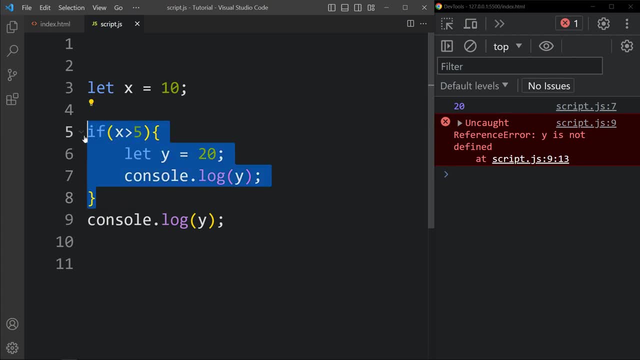 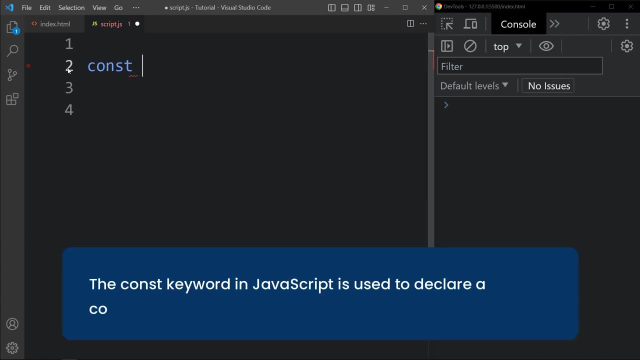 variable y is not defined outside of this block. now let's understand about the const keyword. so the const keyword in javascript is used to declare a constant variable. this means that the variable cannot be reassigned to a new value. for example, if i write const a equal. 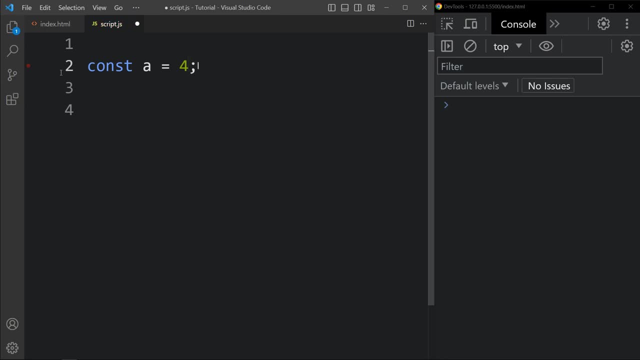 to 4. so we are assigning a value 4 in the a variable. now if i print this console dot log, we will get 4 in the console tab. now in the next line, if i try to write a equal to 5, we are trying to reassign a new value, a equal to 5, and run this, you can see we got an error. 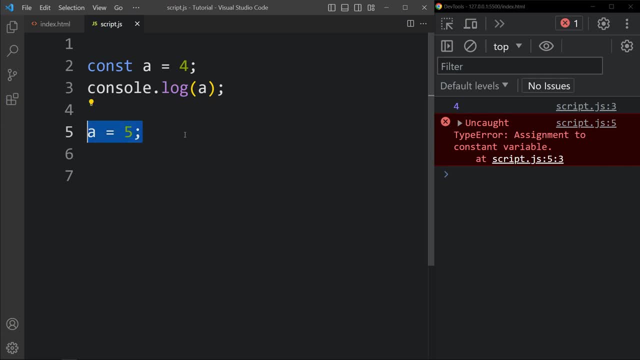 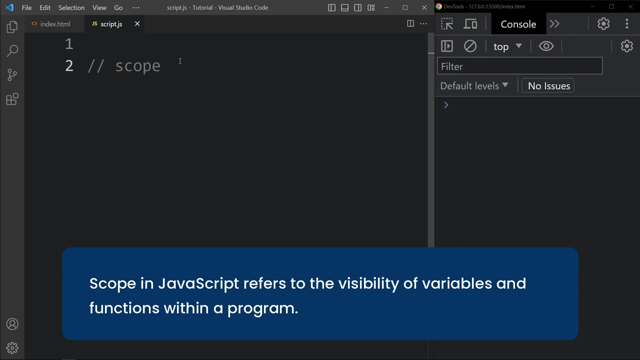 assignment to constant variable. so we cannot assign a new value in constant variable. so let's start with the next line. now let's learn about the scope in javascript. scope in javascript refers to the visibility of variables and functions within a program. in javascript, there are three type of scope. 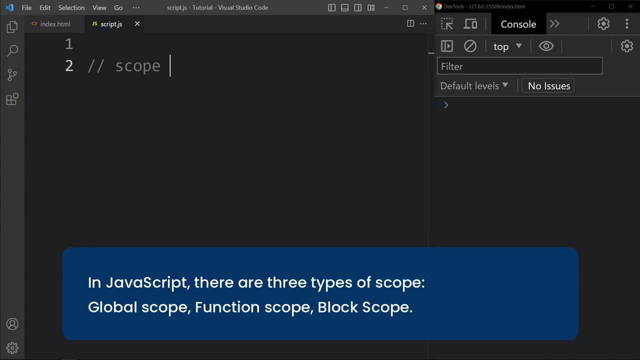 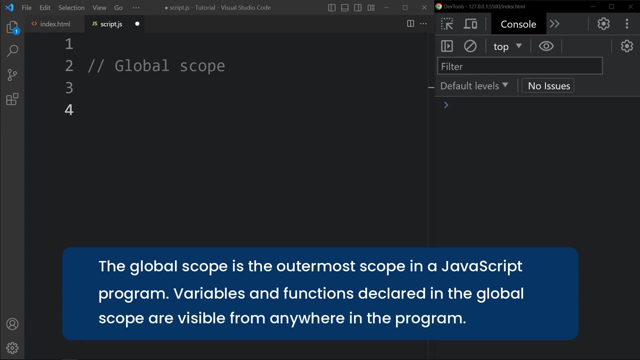 global scope, functional scope and the third one is block scope. so let's learn about the global scope. the global scope is the outermost scope in the javascript program. variables, Examples and functions declared in the global scope are visible from anywhere in the program. Let's understand it with one example. 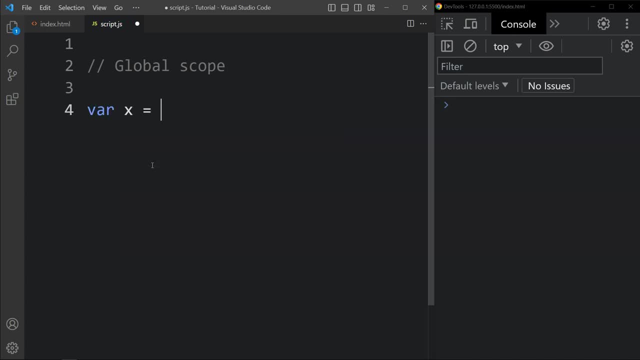 If I write var x equal to hello, great stack. And here we create one function called example, And in this one, if I try to print this message, if I write console dot, log x, And now we have to call this function example. 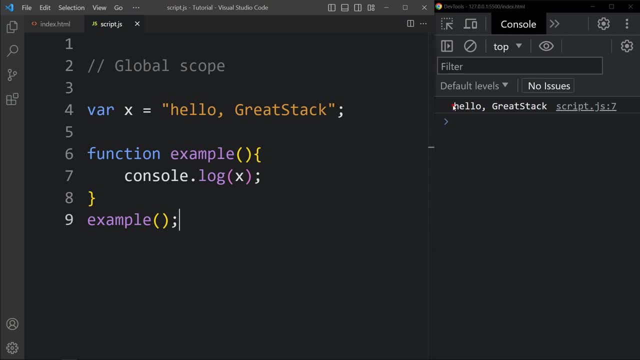 Now you can see This message in the console tab: Hello, great stack over here. In this example, we have declared a variable x outside of any function or block, which makes it a global variable. Global variables are accessible from anywhere in the script, including inside a function. 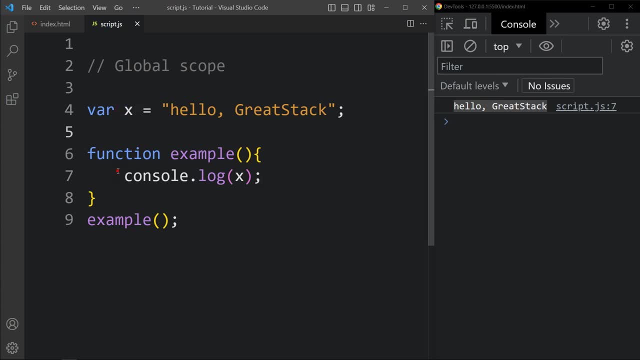 And we have declared this outside of the function, so we can access it within the function and outside of the function also. If I simply Add this here And it will also print this, You can see hello, great stack two times. The first one is printed using this console dot log written inside the function. 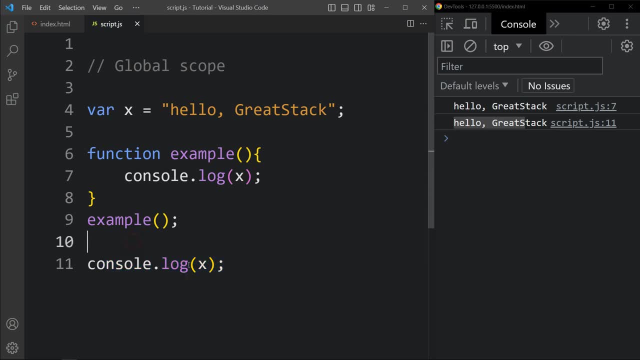 And the second message is printed using this console: dot log x. So this was the global scope. Now let's understand what is the function scope. So, Hello, Great. So the function scope is created when a function is declared, variables and functions declared. 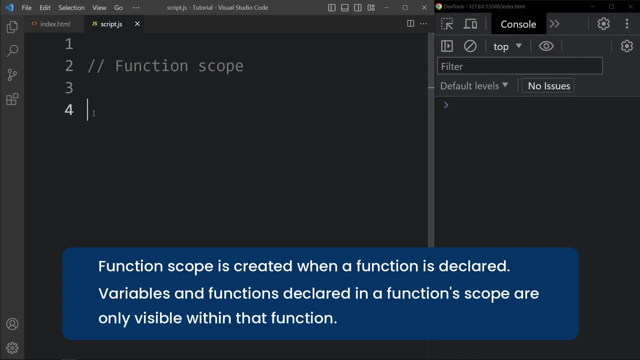 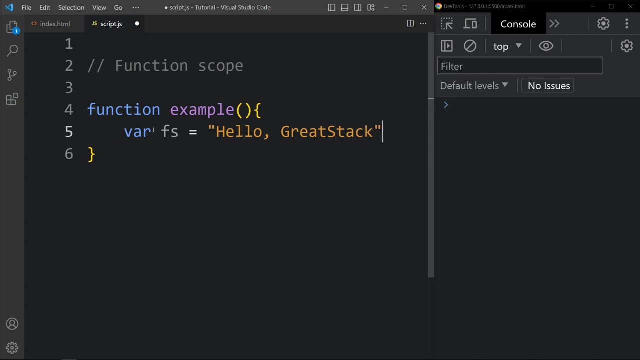 in a functions of scope are only visible within that function. So let's understand this function scope with one example. Here we will add function example. Here we will create one variable Where Fs Function scope equals to: Hello, great stack. 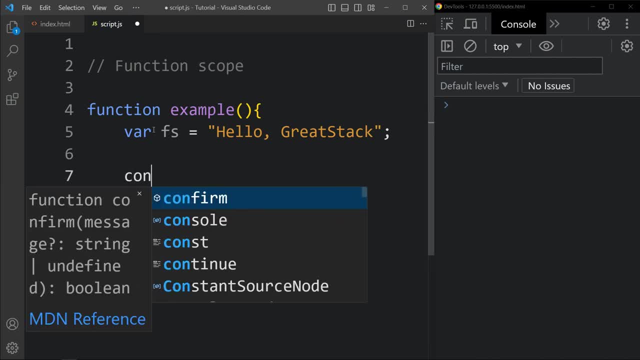 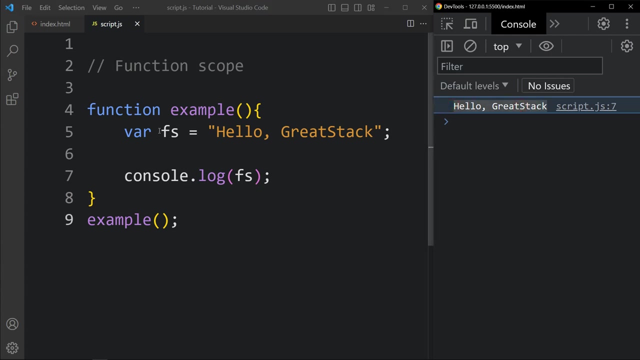 And if I try to display the output, We will add Console dot log Fs And now just Call this function Fs. so now you can see this message: hello, great stack, because we are accessing this variable inside this function. now, if i try to access this fs outside of this function, 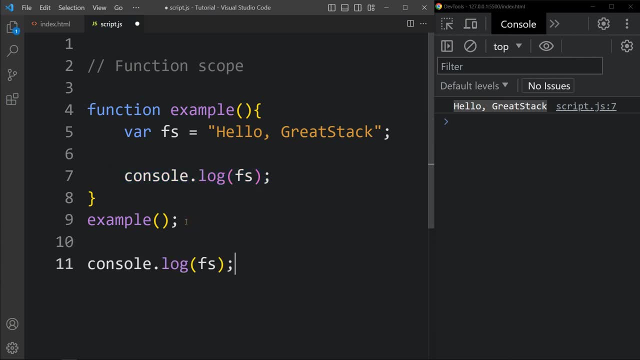 let's copy this and paste it here outside of this function and try to run it. we got an error: fs is not defined. why? because we have defined this fs variable inside this function, so it is a function, a scope variable, and now we are trying to access this fs outside of this function. it is. 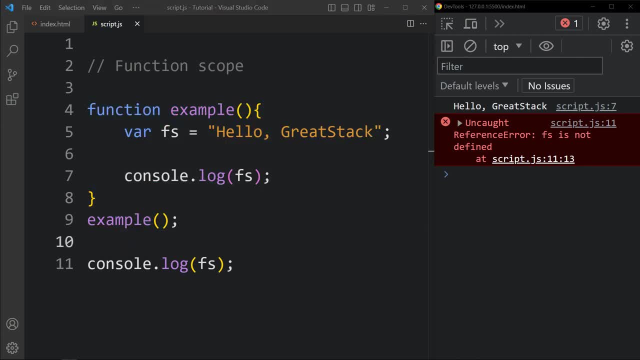 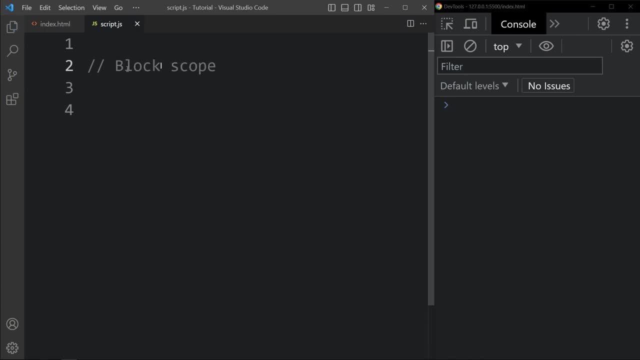 not accessible. so the variables and functions declared in a functions, a scope are only visible within that function. now let's understand the block scope. so the block scope in javascript refers to the visibility of variables and functions within a block of code. a block of code is a group of a statement. 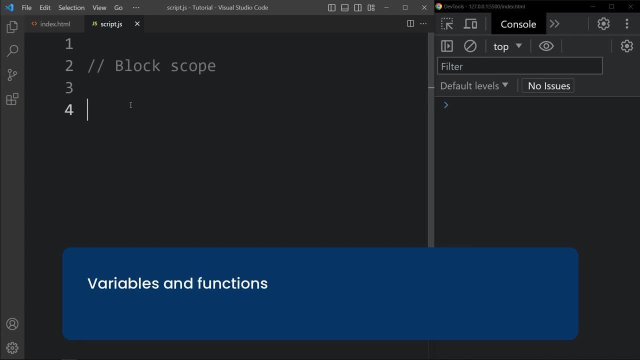 that are enclosed in a curly braces. variables and functions declared in a block scope are only visible within that block. let's understand block scope with one example: let's create one function and in this one we will create one block. true, and here we are creating one block with this curly braces. so within this, if we will add one variable, so let's add the variable. 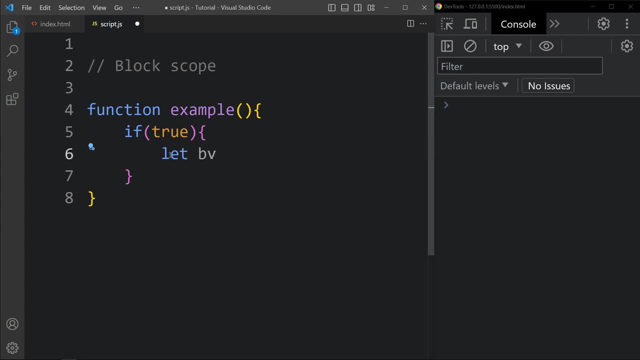 name block variable bv equal to create a stack. and here if we try to display this console dot log bv and just call this example, now you can see this message: great stack in the console tab here because we are accessing this variable inside this block. now, if i try to access this variable, 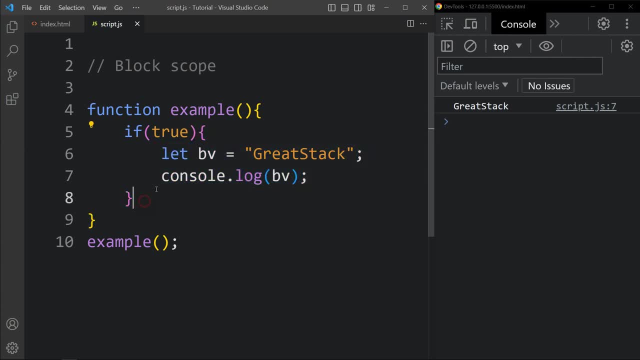 outside of this block. it is declared inside this block and if i try to access here, this block is closing here. so let's add this line here at line number nine. And now, if I try to run, you can see we got an error in line number 9, bv is not defined. 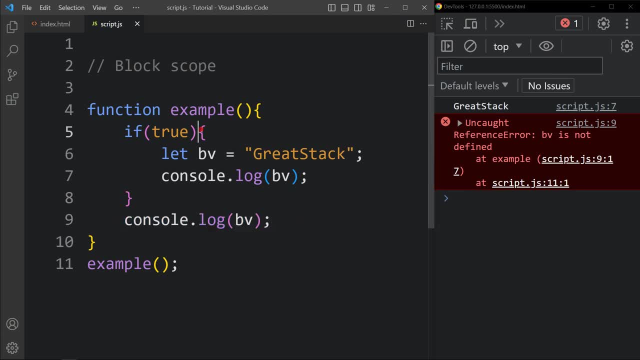 Because we are accessing this variable outside of this block. Let's try to access this variable outside of this function only. Let's remove it from here, add it here at the end, And now you can see the error message at line number 12, bv is not defined. 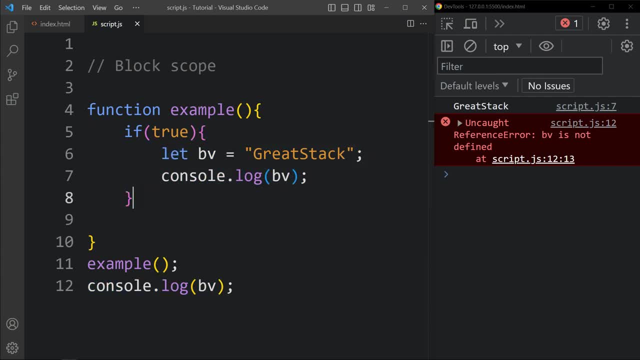 Because we are trying to access this variable outside of this block. So the variable and functions declared in a block scope are only visible within that block. So this was all about the variables and scope in JavaScript. I hope this video will be helpful for you. 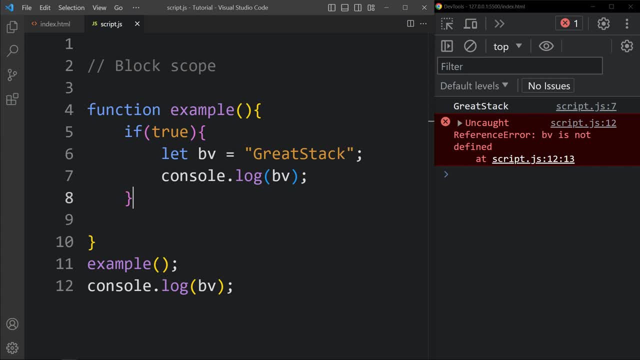 If you have any question, you can ask me in the comment section. Please like and share this video and also subscribe my channel, greatest tech, to watch more videos like this one. Thank you so much for watching this video.